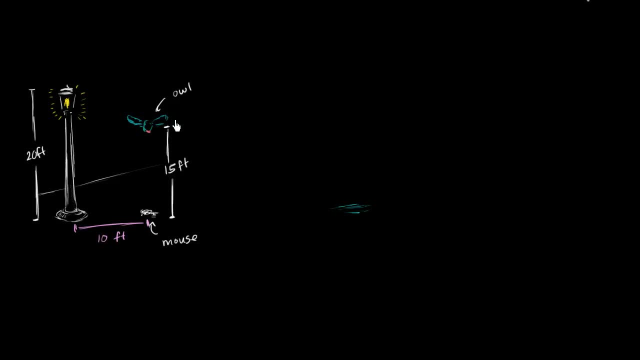 down is driving straight down And right now it is going 20 feet per second. So right now this is going down down at 20 feet per second. Now what we're curious about is: we have the light over here. Light is coming from the 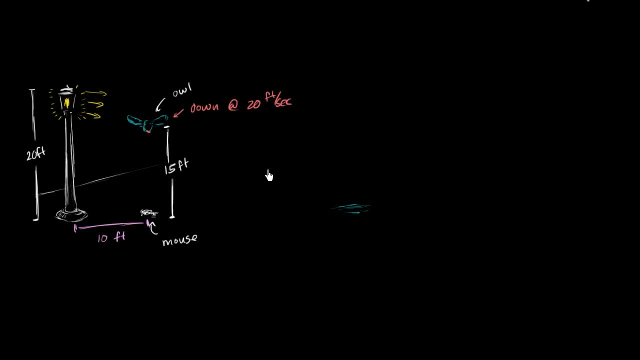 street lamp in every direction And it creates a shadow of the owl. So right now, the shadow is out here And as the owl goes further and further down, the shadow is going to move to the left like that, And so, given everything that we've set up right over here, 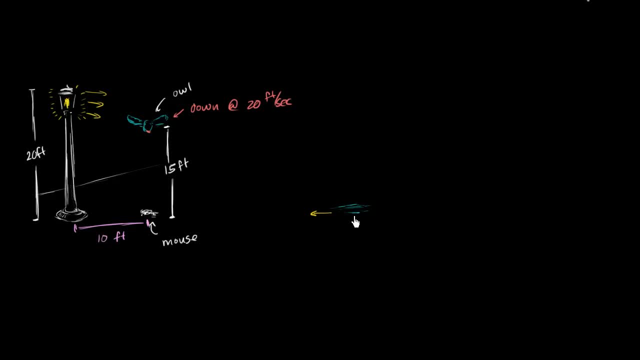 the question is: at what rate is the shadow moving? So let's think about what we know and what we don't know, And to do that let's set up some variables. So let me draw the same thing a little bit more geometrically. 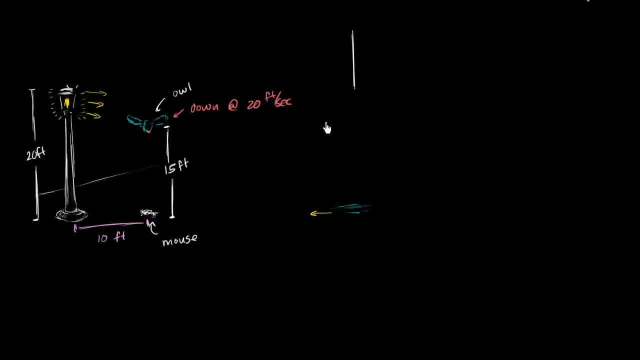 So let's say that this right over here is the street light that is 20 feet tall, And then this right over here is the height of the owl right at this moment. So this is 15 feet, The distance between the base of the lamp. 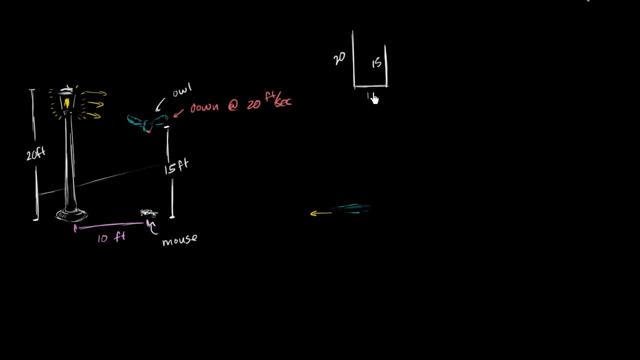 and where the owl is going, where that mouse is right now. this is 10 feet, And if I were to think about where the shadow is, well, the light's It's emitting from right over here. The light's emitting right over here. 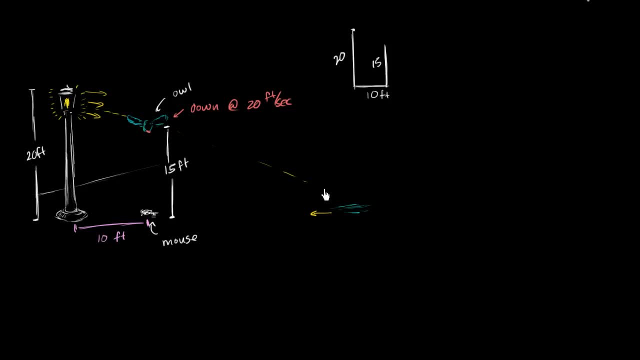 And so the owl blocks the light right over there, So the shadow is going to be right over there. So if you just draw a straight line from the source of light through the owl and you just keep going and you hit the ground, you're going. 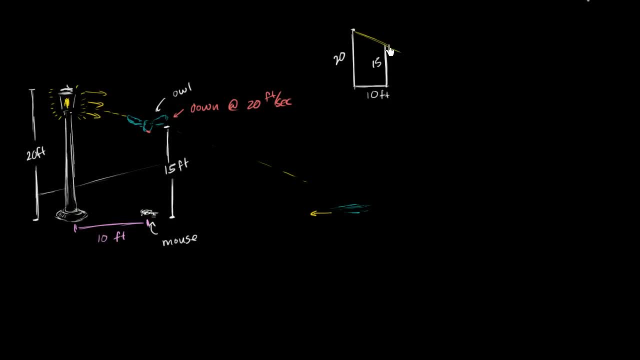 to figure out where the shadow is. So the shadow is going to be right over here. It's going to be right over there And we need to figure out how quickly is that moving? And it's going to be moving in the leftward direction. 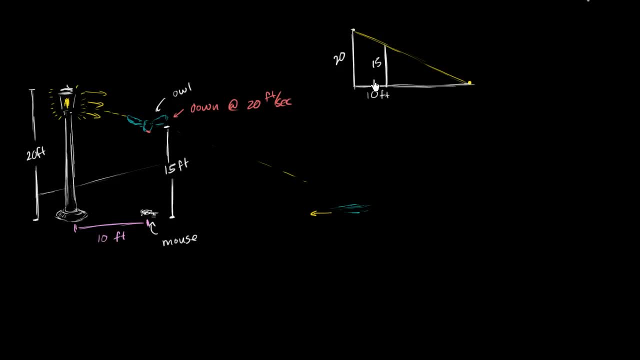 So let's set up some variables over here. So let's say so. what's changing? Well, we know that the height of the owl is changing, So let's call that y Right. at this moment it's equal to 15.. 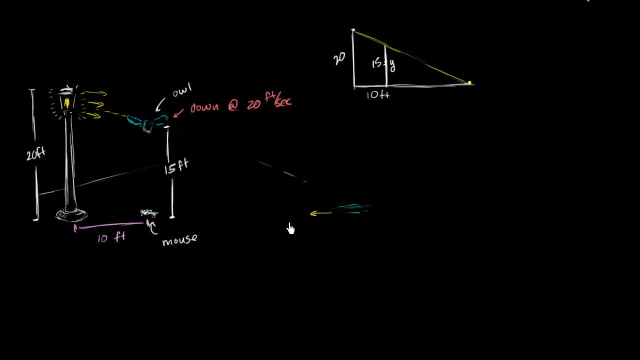 But it is actually changing. And let's call the distance between the shadow and the mouse. let's call that distance x. Now, given this setup, can we come up with a relationship between x and y And then, using that relationship, what we're really trying to come up with? 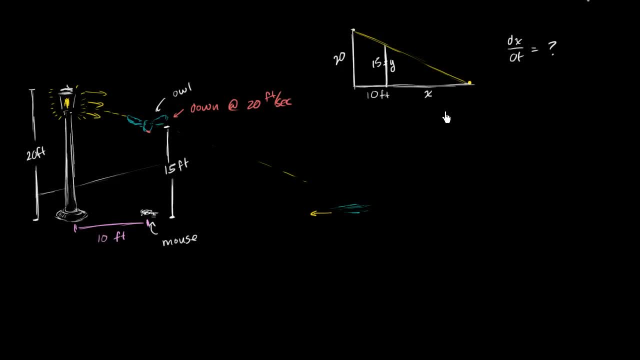 is: what is the rate at which x is changing with respect to time? We know what y is right at this moment. We know what dy, dt is right at this moment. Can we come up with a relationship between x and y and maybe take the derivative with respect to t? 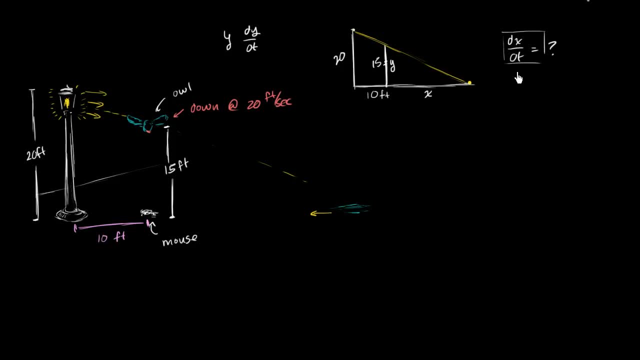 so we can figure out what dx dt is at a given moment in time. OK, Well, both of these triangles. and when I say both of these triangles, let me be clear what I'm talking about. This triangle right over here, this smaller triangle in green: 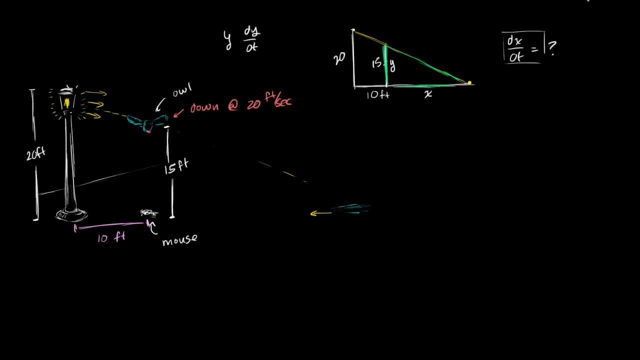 is a similar triangle to the larger triangle is a similar triangle to this larger triangle that I am tracing in blue. It's similar to this larger one. How do I know that? Well, they both have a right angle right over here. They both share this angle. 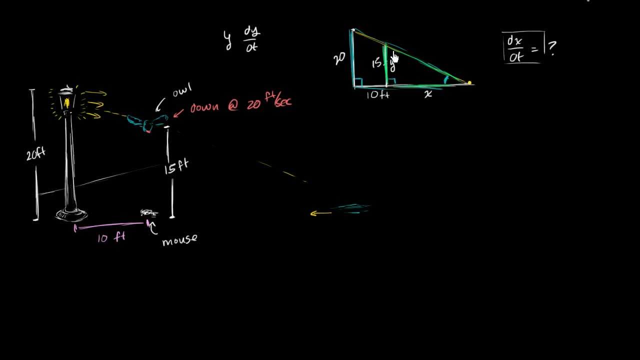 So all three. if they have two angles in common, then all three angles, All three. All three angles must be in common, So they are similar triangles, which means the ratio between corresponding sides must be the same. So we know that the ratio of x to y 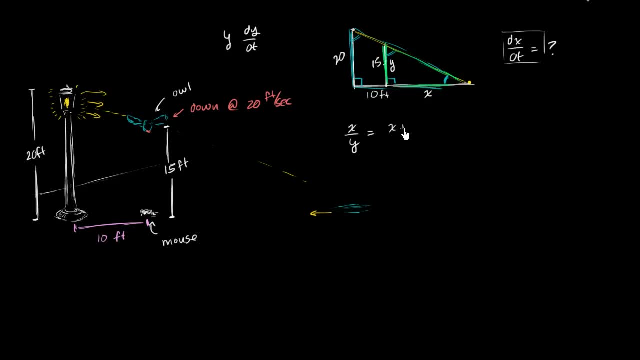 must be the ratio of this entire base, which is x plus 10, to the height of the larger triangle 220.. And right there we have a relationship between x and y, And if we take the derivative of both sides with respect to t, 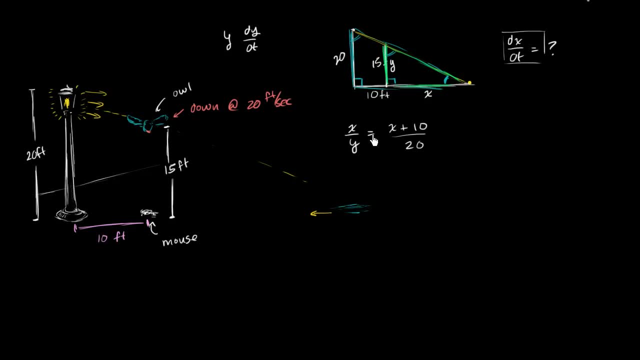 we're probably doing the same thing. We're probably doing pretty well. Now, before taking the derivative with respect to t, I could do it right over here. Just to simplify things a little bit, let me just cross multiply. So let me multiply both sides of this equation by 20 and y. 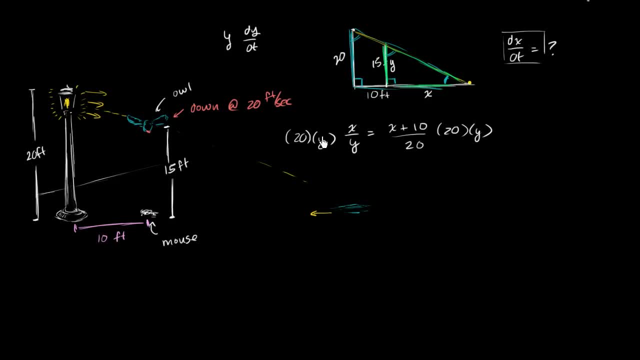 just so that I don't have as many things in the denominator. So on the left-hand side it simplifies to 20x. I don't want to write over it. Well, I'll just write 20x, And on the left-hand side it is 20x. 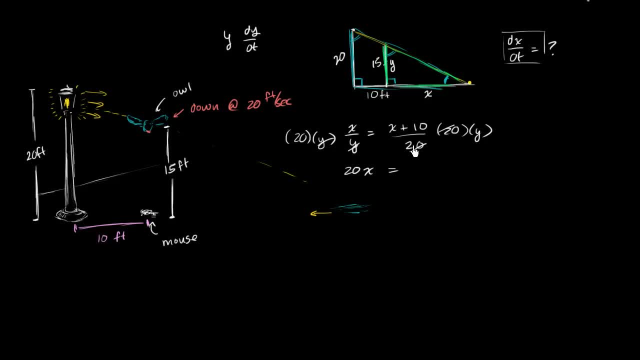 And then on the right-hand side, let's see this cancels. with that We have xy plus 10y, And now let me take the derivative of both sides with respect to time, So the derivative of 20 times something with respect to time. 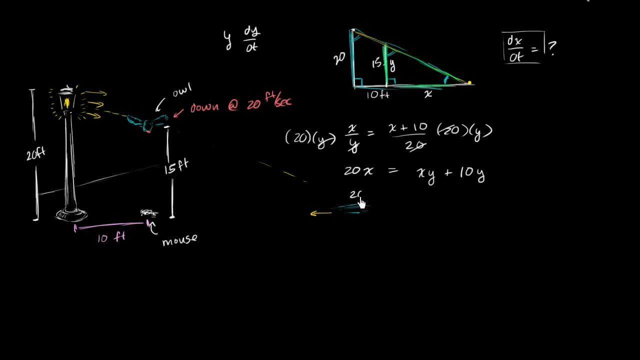 is going to be the derivative of 20 times something with respect to the, something which is just 20.. That's the derivative of 20x with respect to x times dx. the derivative of x with respect to t is equal to. 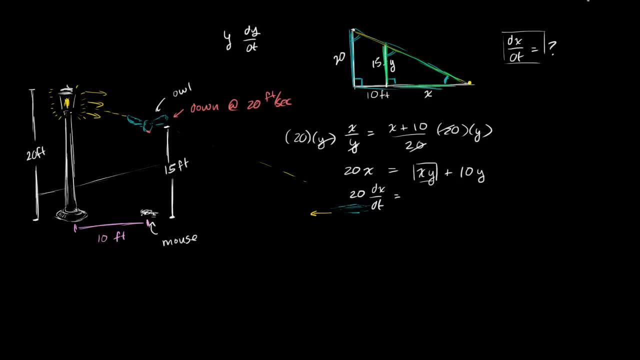 Now over here we're going to have to break out a little bit of the product rule. So first we want to figure out the derivative of x with respect to time. So the derivative of x with respect to time, so the derivative of the first thing times the second thing. 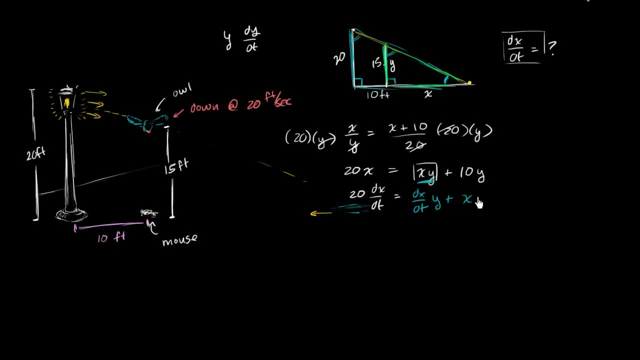 times y, plus just the first thing times the derivative of the second thing. So the derivative of y with respect to t is just dy, dt. And then finally, right over here, the derivative of 10y with respect to t is the derivative of 10y. 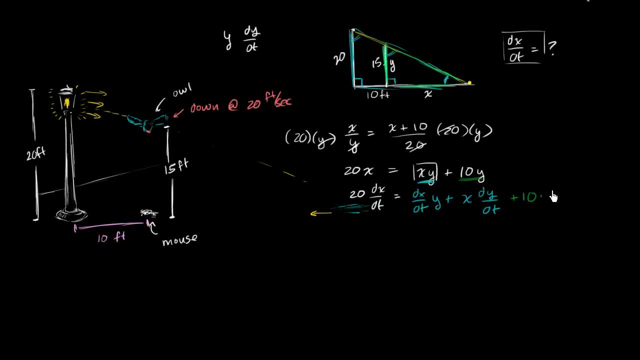 with respect to y, which is just 10, times the derivative of y, with respect to t, which is dy, dt. And there you have it. You have your relationship between dx, dt, dy, dt and x and y. So let's just make sure we have everything. 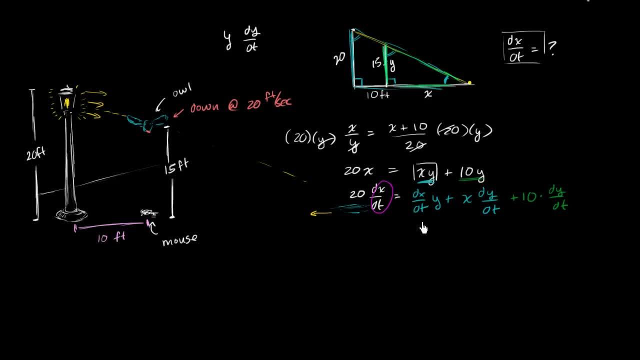 This is what we're trying to solve for dx dt. And let's see, we have another dx dt here We're going to try to solve for that. We know what y is. y is equal to 15.. We know what dy dt is. 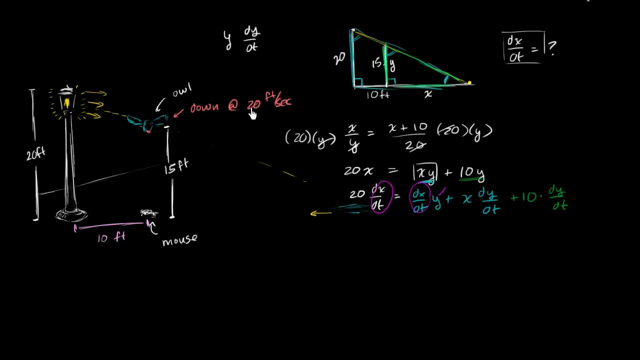 If we make the convention, since y is decreasing, we can say it's negative 20. So we know what this is, And so if we just know what x is, we can solve for dx, dt. So what is x right at this moment? 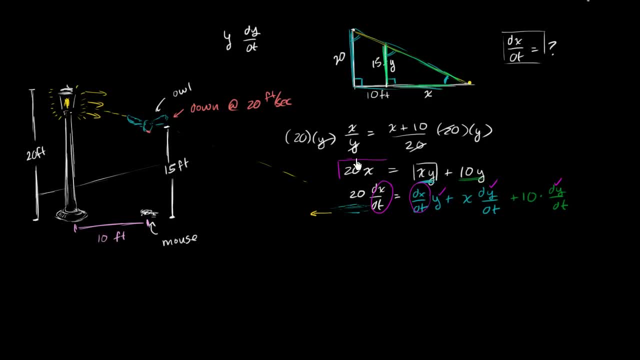 Well, we can use this first equation. We could actually use this one up here, But this one is simplified a little bit to actually solve for x. So let's do that, and then we'll substitute back into this thing where we've taken the derivative. 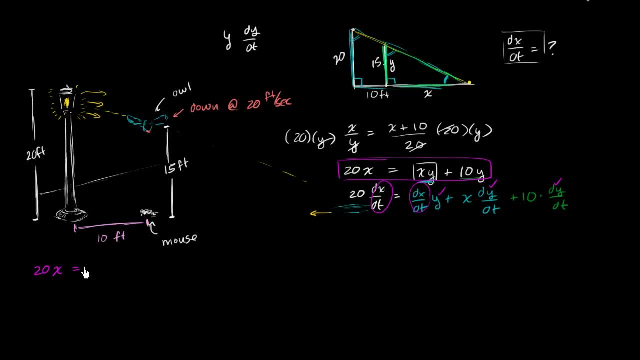 So we get 20 times x. x is equal to x times y, y is 15.. And just remember- I could have used this equation, But this is just one step further- We've already cross-multiplied, So it's x times y. 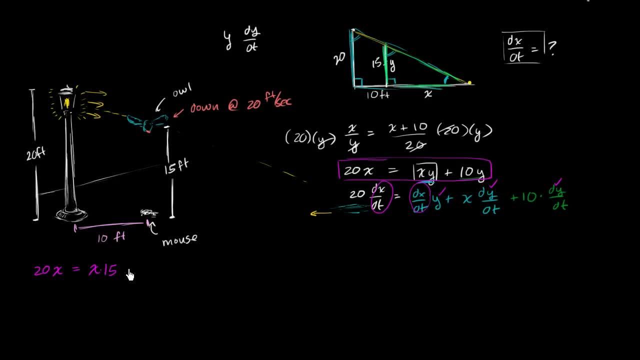 y is 15.. So it's x times 15 plus 10 times y Plus 10 times 15.. Did I do that right? 20x is equal to x times 15 plus 10 times 15.. 10 times 15.. 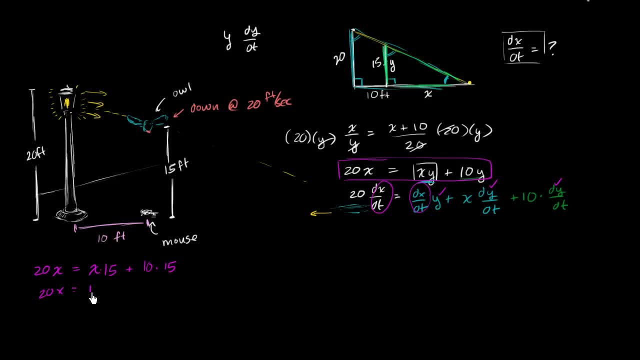 So let's see: If you subtract, So this is 20x, x is equal to 15x plus 150.. Subtract 15x from both sides, You get 5x is equal to 30.. Divide, I'm sorry. 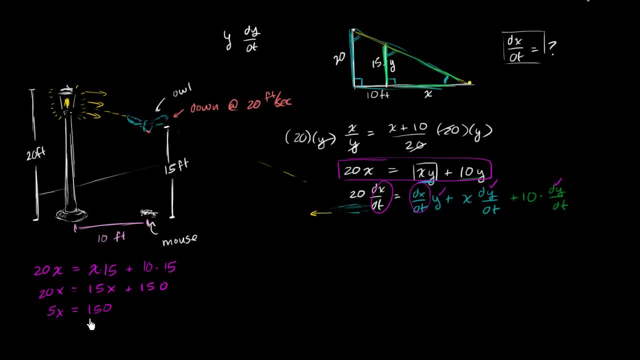 5x is equal to 150.. My brain is getting ahead: 5x is equal to 150.. Divide both sides by 5.. You get x is equal to 30 feet. x is equal to 30 feet right at this moment. 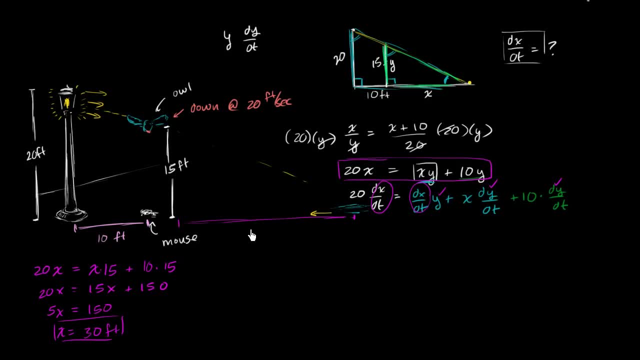 So this distance, just going back to our original diagram, this distance right over here is 30 feet. So let's substitute all the values we know back into this equation to actually solve for dx, dt. So we have, so let me do it right over here. 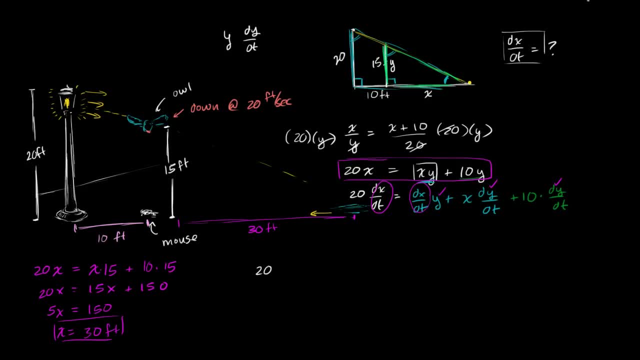 We have 20 times dx dt. I'll do that in orange. We'll solve for that. Actually I already used orange, So let's say dx dt. I'll use this pink. 20 times dx dt is equal to dx dt times y. 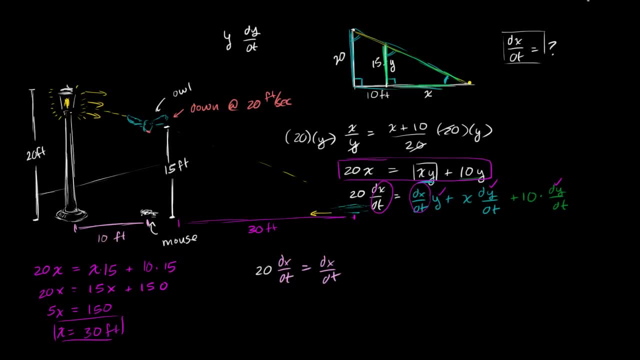 y right now is 15 feet, So times 15. 15. 15. 15. 15.. I didn't want to do that. color Times: 15 plus x. We already know that x is 30. Plus 30 times dy dt. 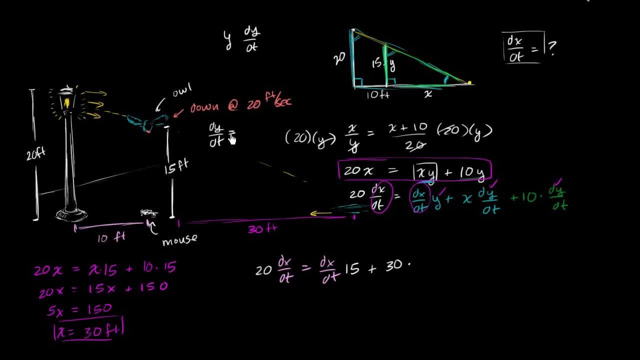 What is dy, dt, dy dt, we could say, is negative: 20 feet per second. y is decreasing. The bird is diving down to get its dinner, So times negative and that's just a well times 20 feet per second. 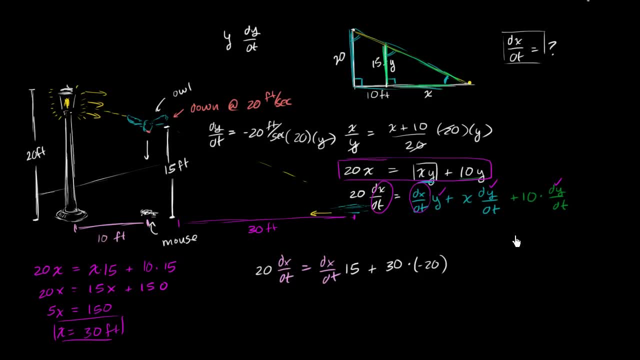 So that's that right over there, Plus 10 times dy dt. So plus 10 times negative 20 feet per second. And now we just solve for dx dt. So let's see What do we have? We have 20 times. let's see: